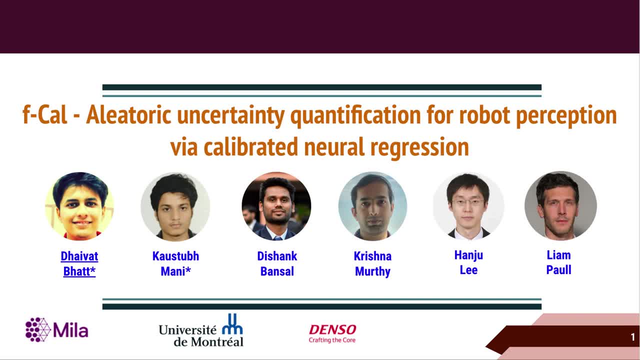 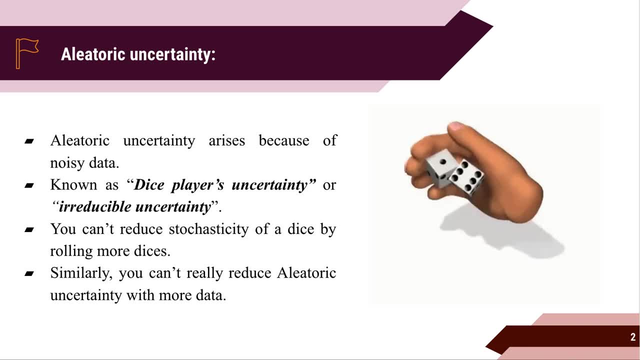 Hi everyone, my name is Dahebar Bhatt. In this work we present F-CAL, a calibration method proposed to train probabilistic neural regressors, Aleator. uncertainty is inherent in the data and it cannot be reduced. It can only be estimated. In this work we aim to obtain 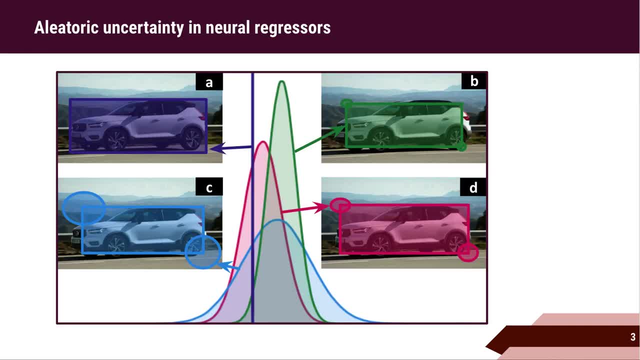 calibrated estimates of aleator uncertainty. In this illustration we see a grounded bounding box in Figure A. Figure B shows an overconfident prediction as denoted by small ellipses. Figure C shows underconfident and highly inflated uncertainty estimate which is consistent in terms. 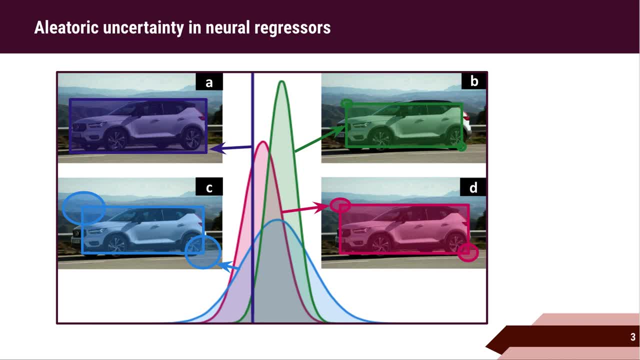 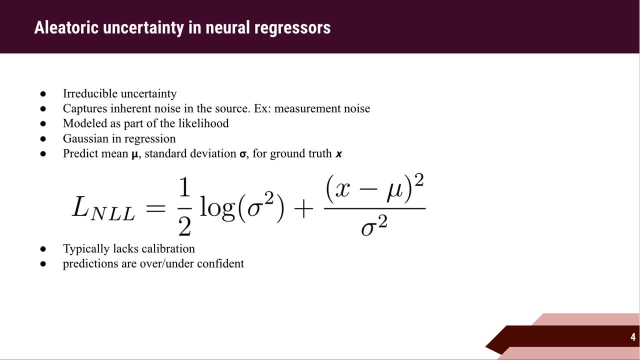 of probabilistic prediction, but not calibrated. Figure D shows correct uncertainty estimate reflecting variance of underlying data distribution. In typical probabilistic neural regressors. aleator uncertainty is modeled as Gaussian distribution and negative log likelihood of Gaussian is used as the objective function to train the neural regressor. 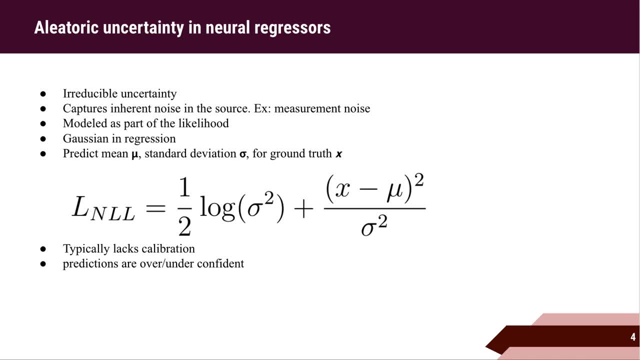 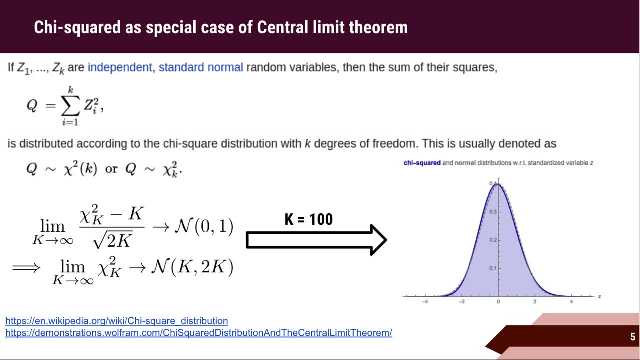 Predicted uncertainties are generally over- or underconfident and they lack calibration. In this work to enforce distribution and calibration constraints, we fuse a set of k-standard normal random variables to create a chi-squared random variable For k greater than 50, the chi-squared distribution converges to Gaussian distribution according to: 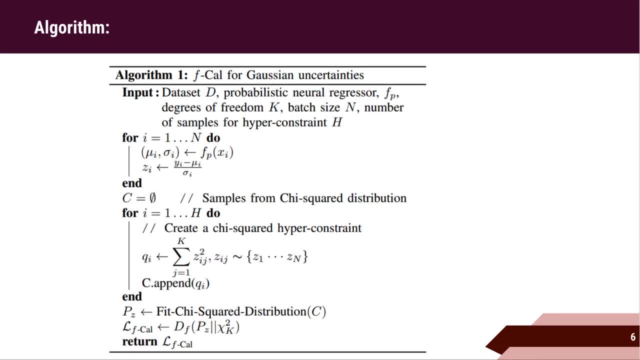 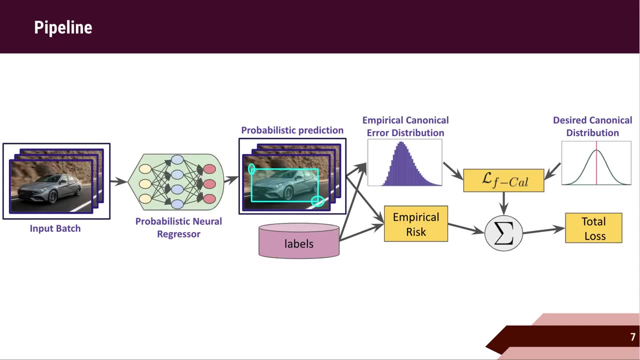 central limit theorem. In our algorithm, a neural regressor predicts mean and standard deviation for an input and we calculate residuals and create chi-squared hyper constraints. We have divergence to match it with the desired target distribution. Given a batch of input data, the model predicts mean and corresponding uncertainty, standard deviations. 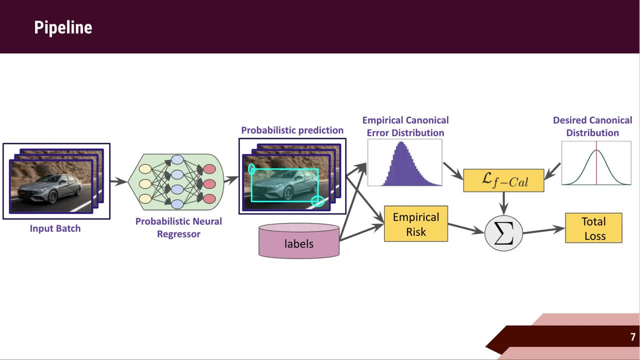 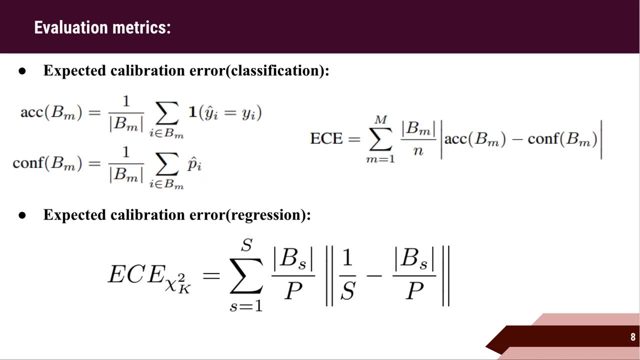 We calculate empirical loss, such as mean squared error or smooth L1, as well as distribution matching loss. to enforce calibration and train the model. To evaluate calibration performance, we use expected calibration error, Expected calibration error or expected calibration error. Z evaluates whether a sample 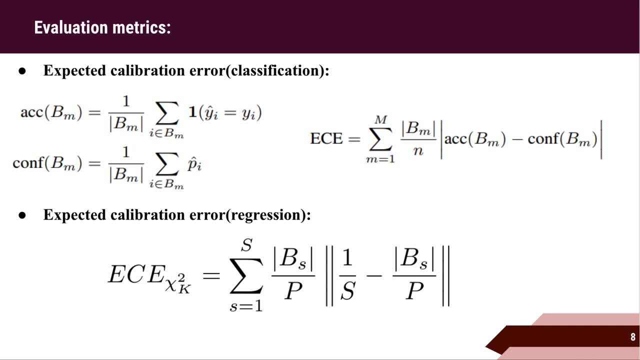 prediction follows a Gaussian distribution or the residual follows a standard normal distribution, And ECE- chi-squared, also denoted as ECEQ, evaluates whether a collection of sample predictions in a batch collectively follow a chi-squared distribution as a result of central limit theorem. Now we present quantitative results of FQL. We compare FQL against various